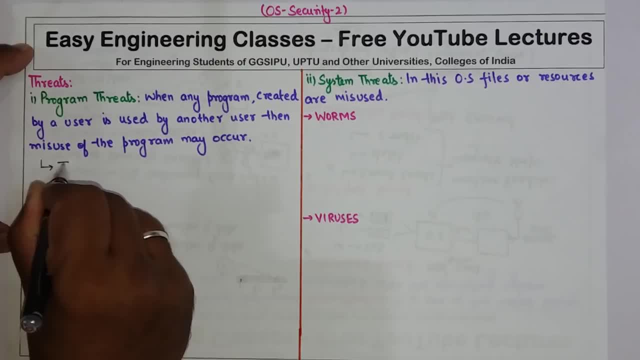 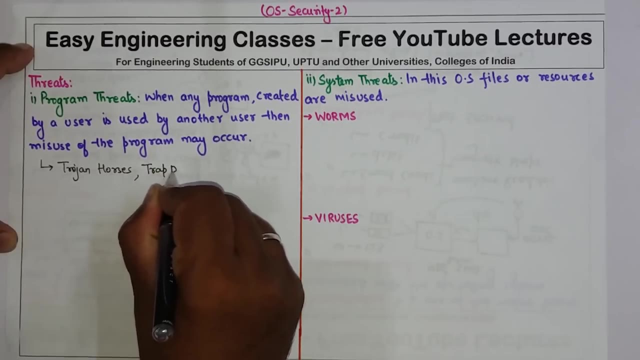 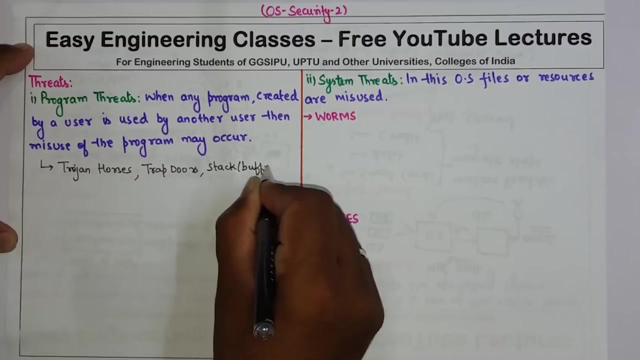 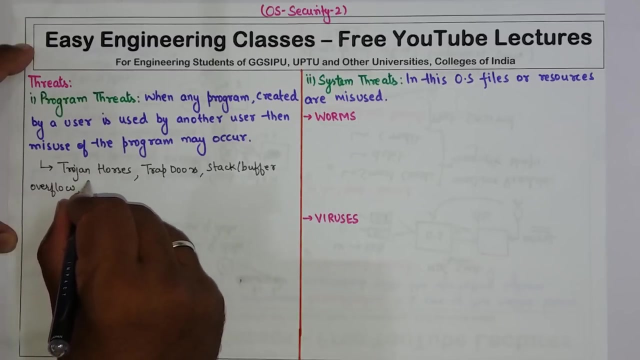 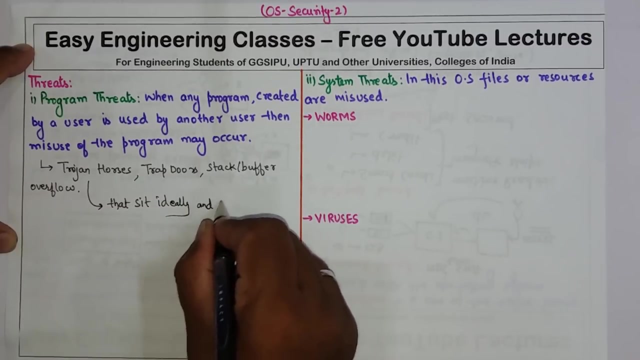 can be achieved are Trojan Horses. Now, these are some of the examples of these program threats Trojan Horses, then we can have Trapdoors, Stack and Buffer Overflow, etc. So if we say that Trojan Horses, Trojan Horses are the programs that sit idly and transmits. 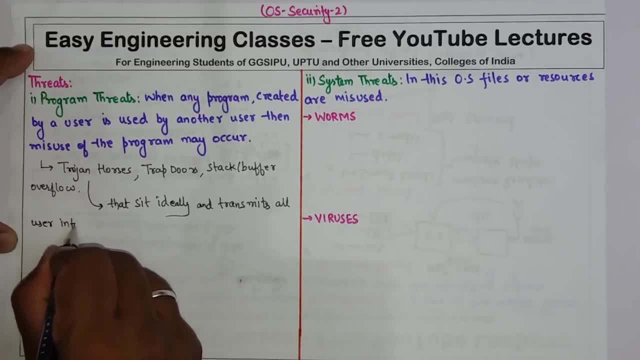 all the user information to the attacker. Now, for example, if there is a Trojan Horse in your system and you are login into your account on any browser and that Trojan Horse is attached to this browser, So whenever you are typing anything like the username and password to any website to access that website, 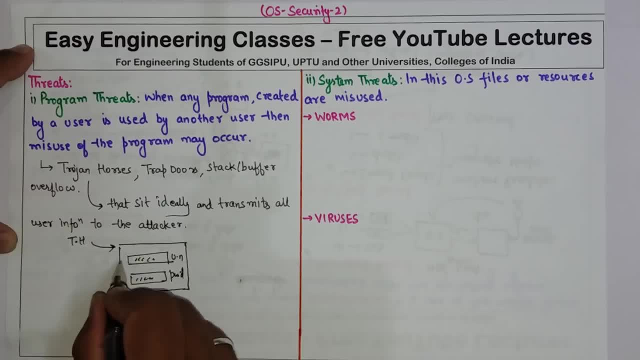 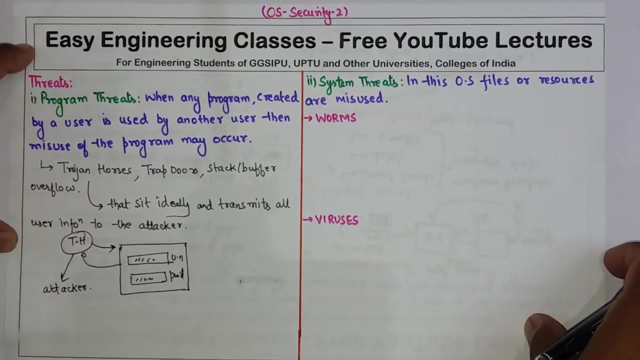 So these information, These information Are recorded by this Trojan Horse and these information are sent to the attacker. In this way, this program, this Trojan Horse program, is created by a user and is used by the attacker to prevent some attacks to the system. 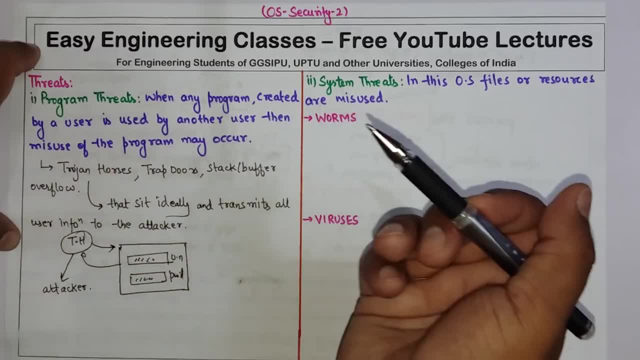 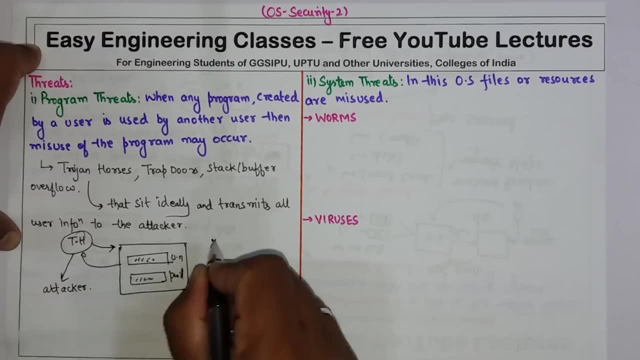 So such kinds of attacks, such kinds of threats come under the program threats. So one more example can be: There is a program created by a user, say X, and that programs get installed on Y's machine. So the program that X created is such that it consumes all of the resources of Y. 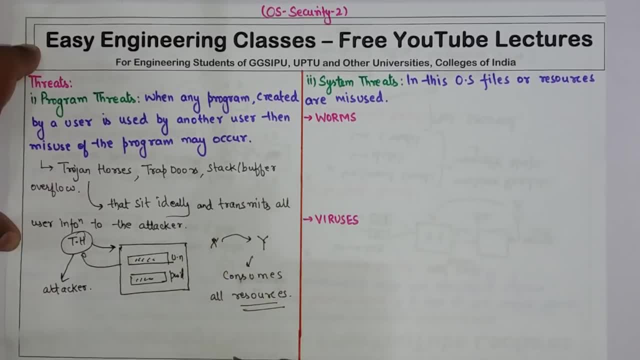 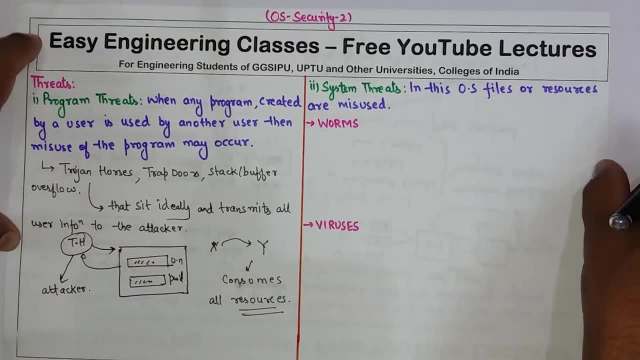 In this kind of situation the buffer overflow can occur. So these are the program threats. So in this kind of situation the buffer overflow can occur. So these are the program threats. So what is the system threats? Then we have system threats. 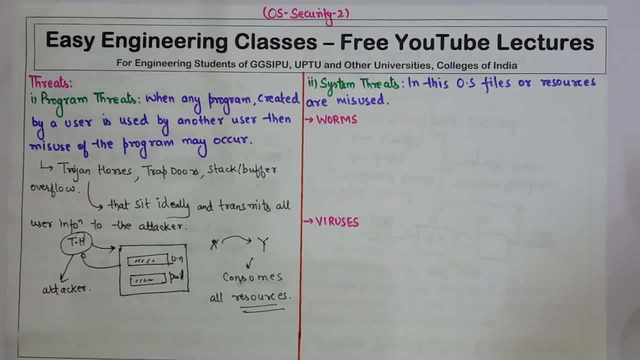 System threats means the OS files or resources are misused. Basically, there are two different kinds of threats to a system: One is worms And another is virus. So what I am going to do is I will write the definition of the theoretical part of this- worms- in. 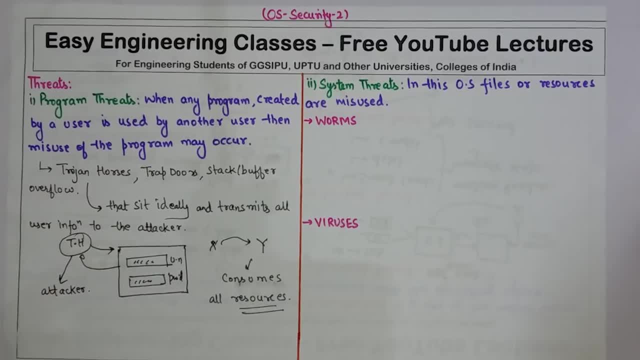 virus and then come back to the video and explain each of this one by one. So worms are the small computer programs that replicates, Or does the machine that replicates One or two of these viruses titles, or least fact That language. 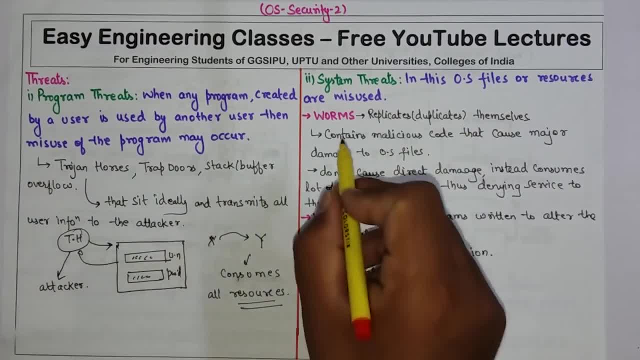 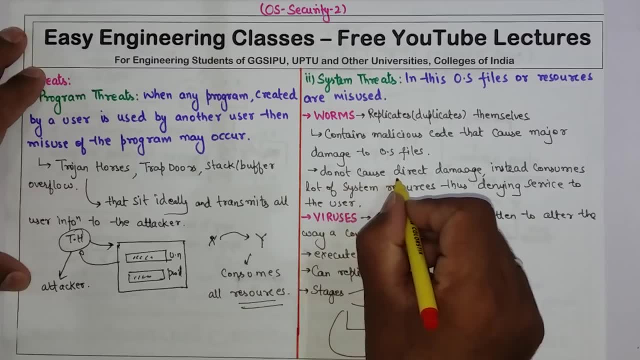 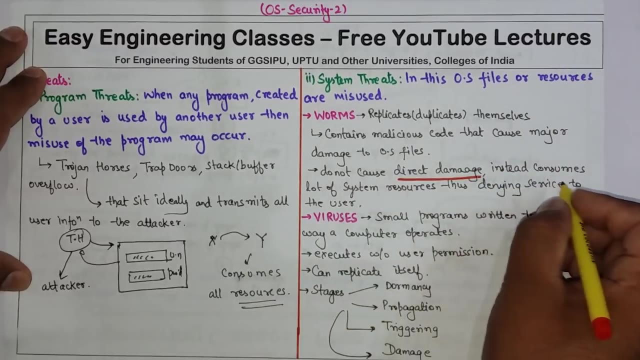 Or fed ф. So there are several fabri duplicates themselves. These worms contains malicious code that cause major damage to the OS files. Now, the worms don't cause direct damage. It is not like that worm deletes a file or do some modification to the files. Instead, they consume lot of system resources, thus denying service to the user. So, for example, if there is a OS and most of the resources of the OS is consumed by worms, So if there are user u1 making some request to the OS, then this service is rejected by the OS because OS resources are itself consumed by the worms, Then viruses 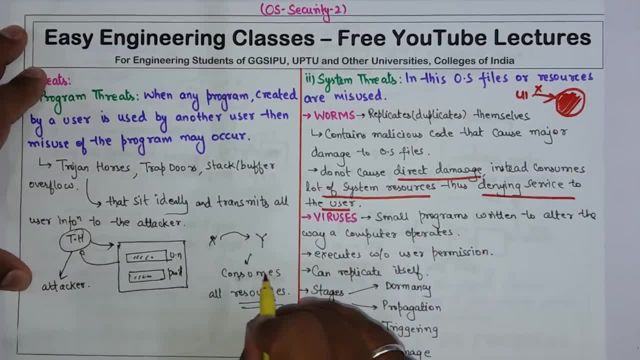 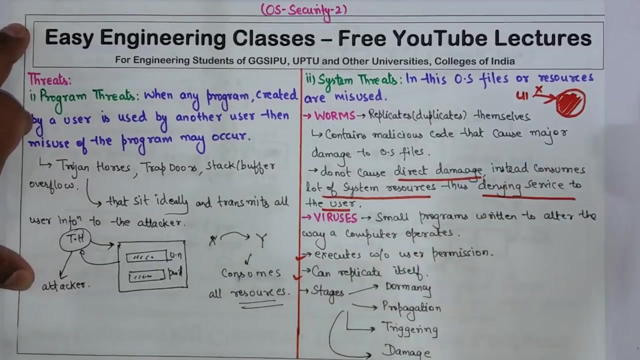 Viruses are small programs written to alter the way a computer operates. Now virus are small programs that replicates itself and also they do some modification to the system files They executes without the user permission can replicate itself, just like worms, but they do certain modification to the files or they change the functionality of the files. Now there are 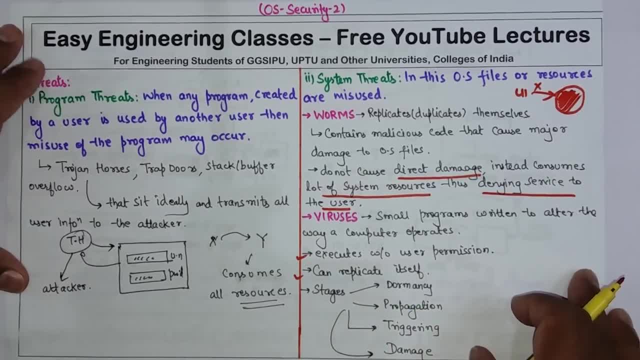 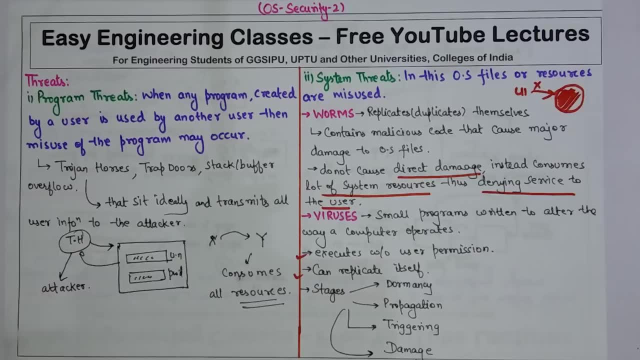 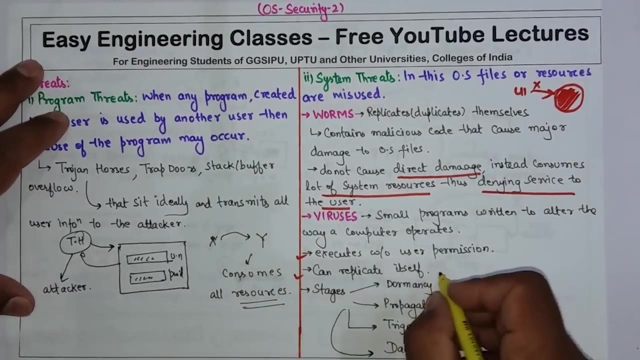 four stages in which a virus can be present. First is the dormancy phase. So on infecting a new machine or a program, a virus remains dormant for a while. Now, dormancy phase is a normal phase in which a virus is present. The dormancy phase means the virus is not doing. 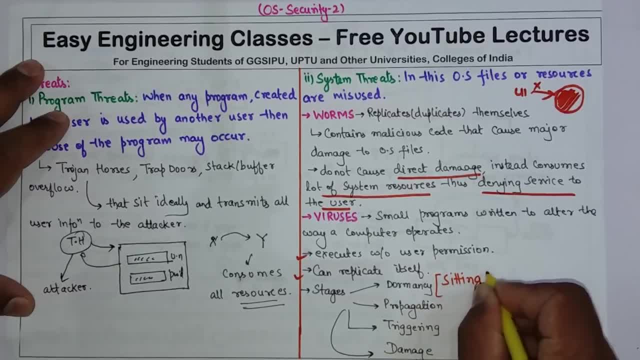 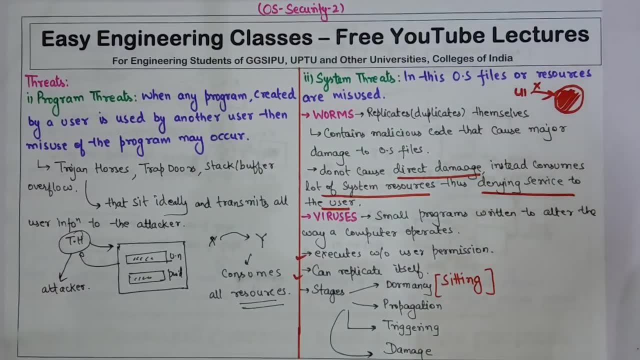 anything, It is just sitting on the system. So, computer it is done. it is done so that the system doesn't detect the presence of the virus in your system. So once the dormancy phase is completed, the virus enters into the propagation phase and in this virus attempts to infect other programs.